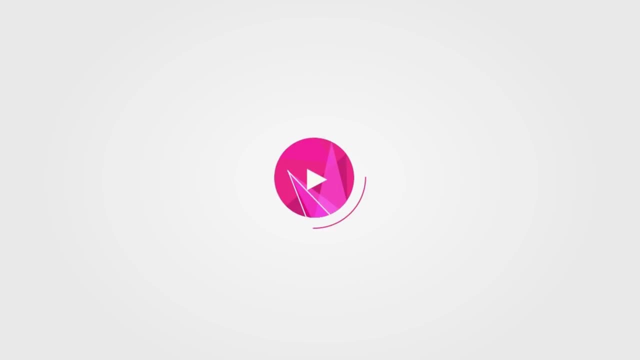 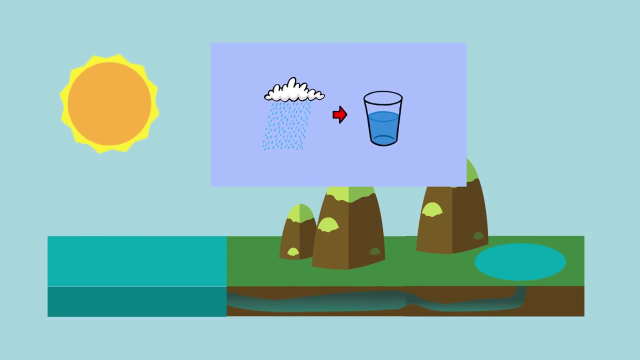 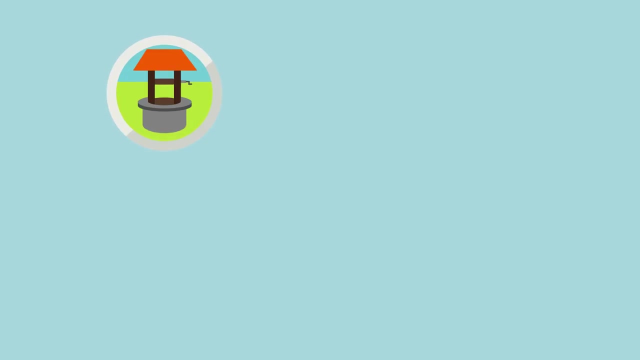 In this video we will see how human beings have added to the natural water cycle. you can see that in one of our linked videos. by taking water from rivers for our use in towns and cities, Humans began to interfere with the natural water courses long ago. Wells have been dug to access clean water for 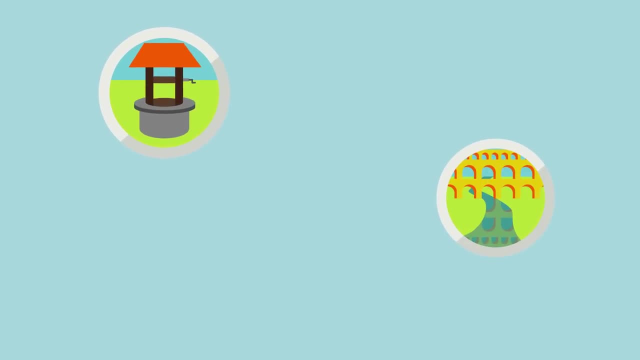 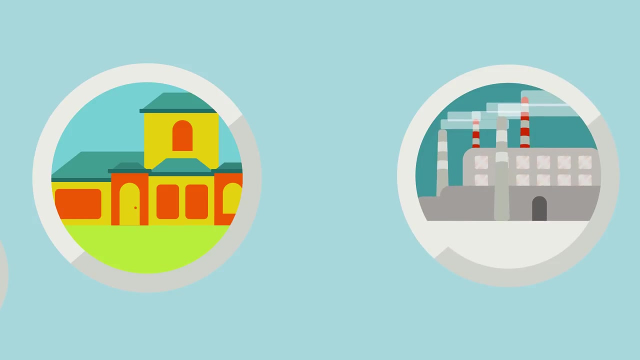 drinking. the Romans built aqueducts to bring water to their cities, and nowadays we've built dams for irrigation and hydroelectricity and we are taking a huge amount of water from natural sources to use in our homes and industries. Most people in industrialized nations take access to clean water for 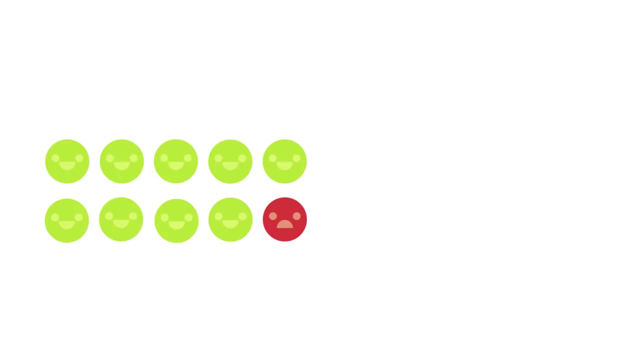 granted. however, more than one person in ten- that's over 700 million people- do not have access to clean water and around three and a half million people die each year from water-related disease. The average Briton uses a hundred and fifty litres a day, whilst each American uses 600 litres a day on average In. 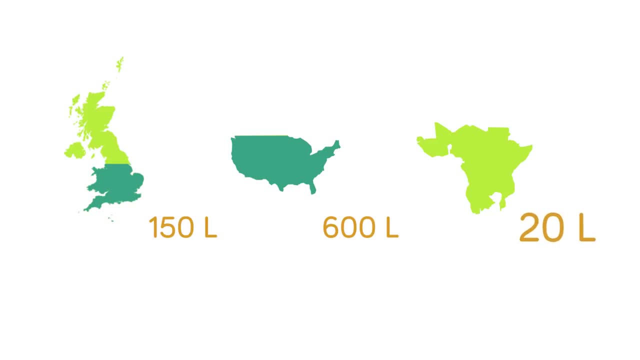 contrast, many sub-saharan Africans get less than 20 litres of water a day, and two-thirds have no proper toilets. For some people, water is a precious and scarce resource. Only three percent of the water in the world is fresh. Of this, three-quarters is 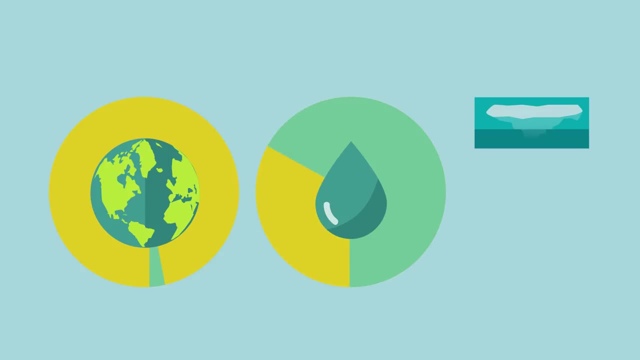 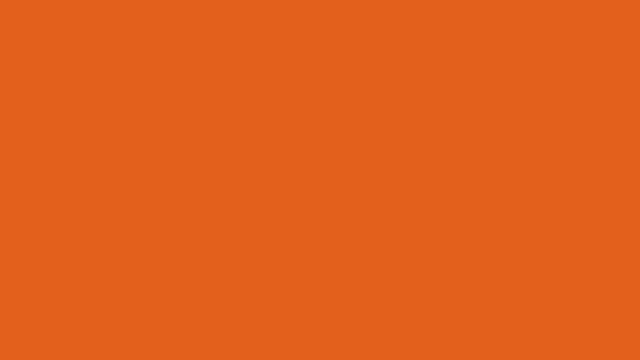 locked up as ice in Antarctica and Greenland and glaciers. Nearly another quarter is underground. Only one percent is above ground in rivers and lakes. We use the water mainly for irrigation of crops and normally this needs no further purification. The next biggest user is industry, Sometimes, for example, in food. 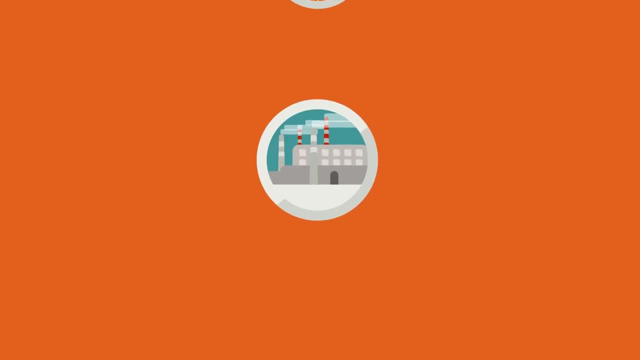 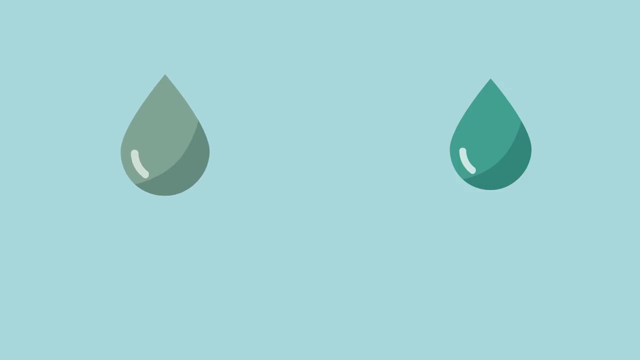 preparation, very clean water is needed. Finally, there is domestic water. Some new housing estates in industrialized countries have a dual water supply, where gray water collected from rain and effluent from basins, baths and showers is available for flushing and. 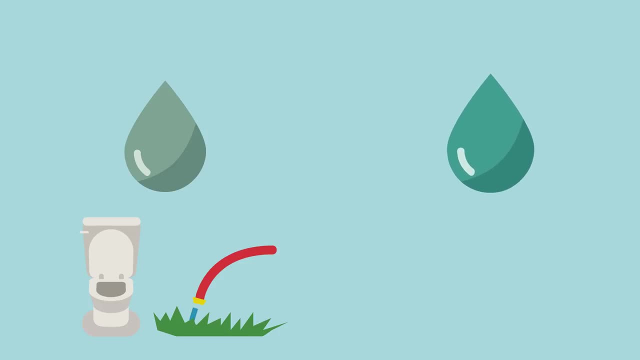 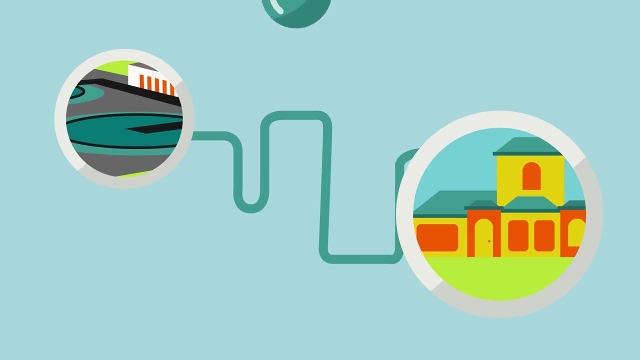 watering the garden, and the purified water is only used for washing and cooking. However, normally only one pipe supplies water to our homes, and this water has to be of drinking quality and is purified on an industrial scale and at the waterworks. If you do not have piped water where you live, you might have access.